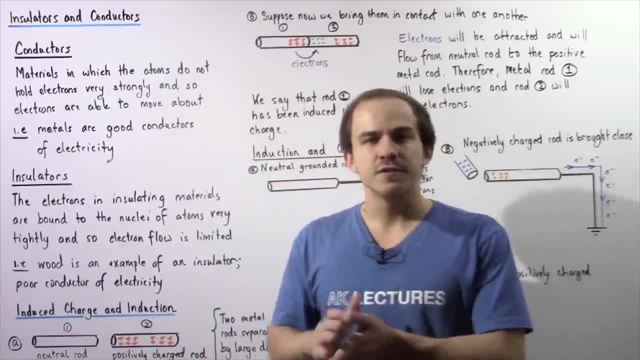 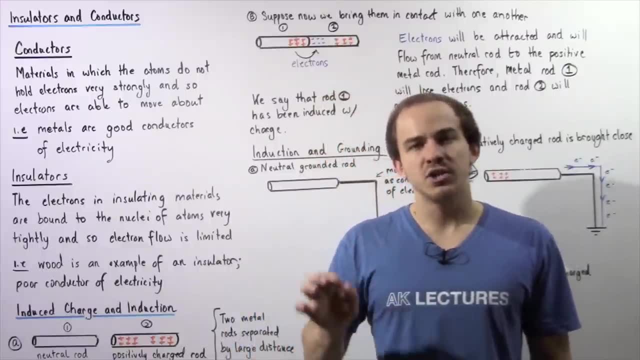 that we have conservation of energy, we also have conservation of energy. So in the same way that we have conservation of energy, we also have conservation of energy. So in the same way that we have conservation of energy, we also have conservation of electric charge. That basically means electric charge cannot be destroyed, nor can 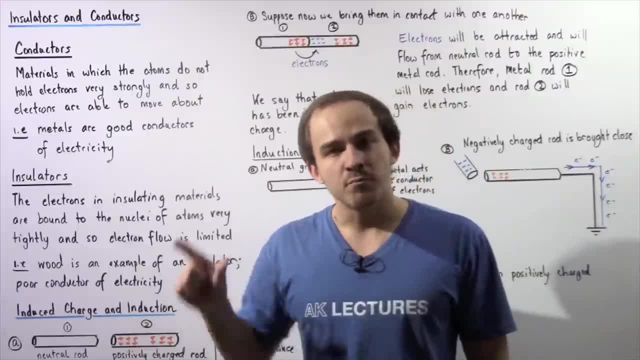 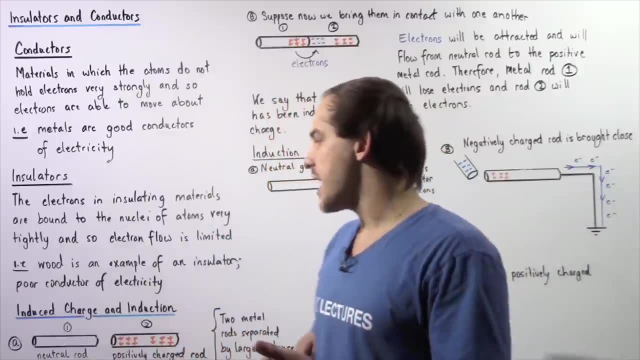 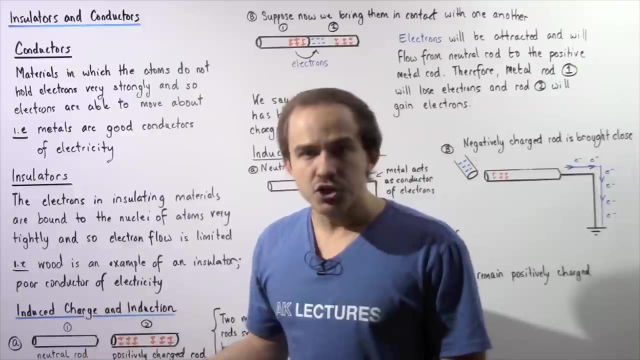 it be created. but electric charge can flow from one object to another object in the same way that energy can flow from one area to another area. So now we're going to essentially discuss a process known as induction and charging objects by induction. So let's suppose we have two objects. 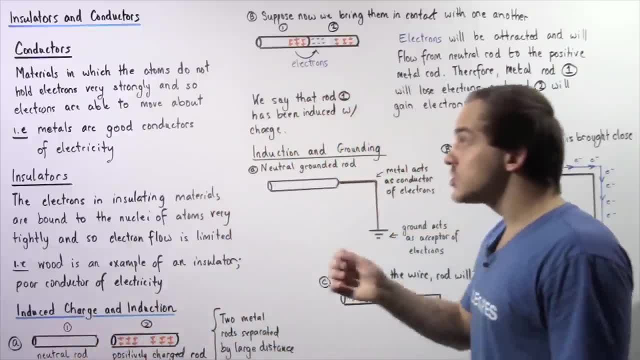 known as induction and charging objects by induction. So let's suppose we have two objects known as induction and charging objects by induction. So let's suppose we have two objects. let's suppose our two objects are metal rods, so that let's suppose we have two objects are metal rods, so that 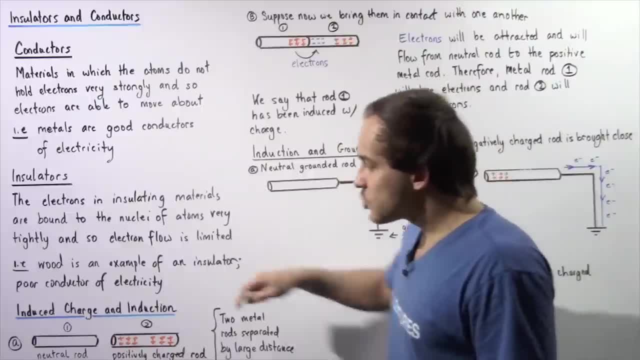 let's suppose we have two objects. are metal rods, so that means they're good conductors of electricity. are metal rods, so that means they're good conductors of electricity. are metal rods, so that means they're good conductors of electricity. So rod number one is a neutral rod. 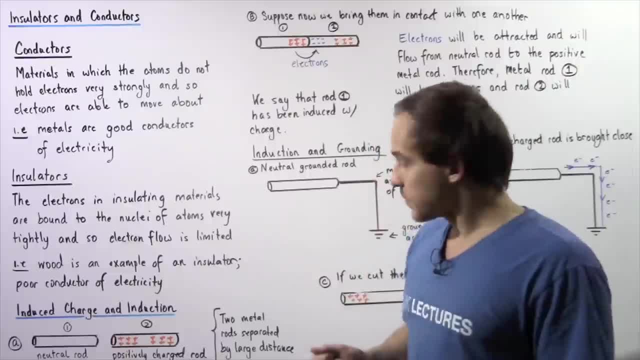 means they're good conductors of electricity. So rod number one is a neutral rod means they're good conductors of electricity. So rod number one is a neutral rod and rod number two has a positive charge. so So rod number one is a neutral rod and rod number two has a positive charge. so 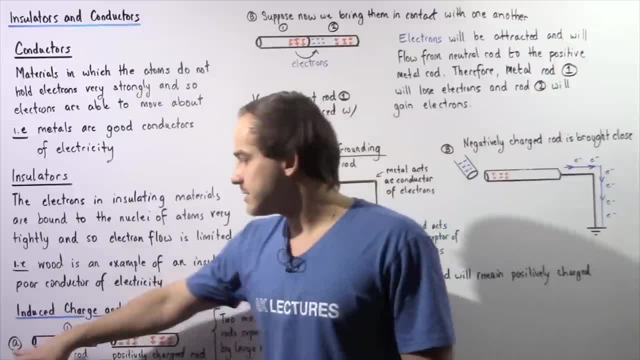 So rod number one is a neutral rod and rod number two has a positive charge. so these two rods are separated by a large and rod number two has a positive charge. so these two rods are separated by a large and rod number two has a positive charge. so these two rods are separated by a large distance in part A. Now if we move to, 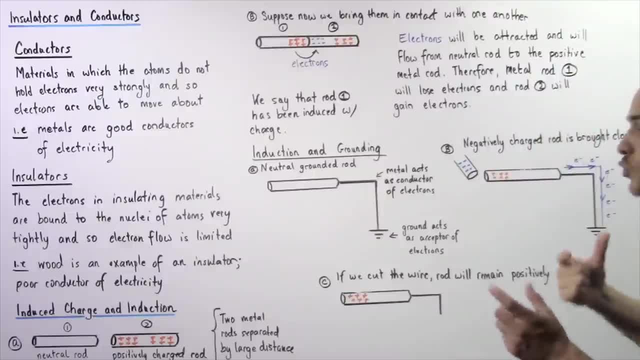 distance in part A. Now, if we move to distance in part A. Now if we move to part B, let's suppose now we bring our two part B. let's suppose now we bring our two part B. let's suppose now we bring our two rods in physical contact with one another. 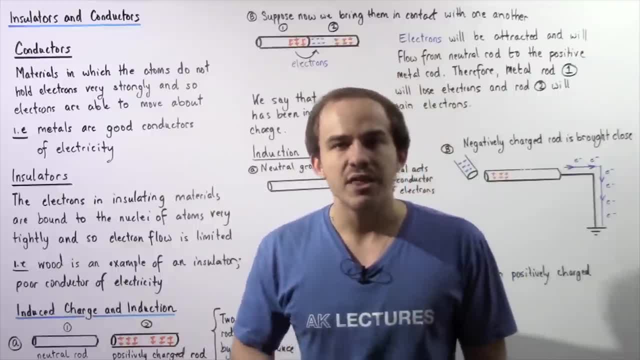 rods in physical contact with one another. rods in physical contact with one another. What will begin to take place? Well, in the. What will begin to take place Well in the. What will begin to take place, Well, in the same way that energy flows from a higher. 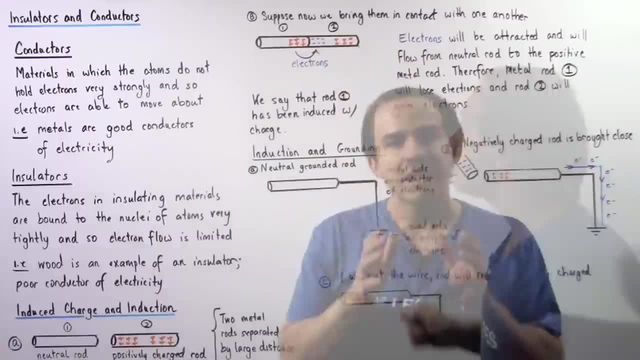 same way that energy flows from a higher, same way that energy flows from a higher temperature to a lower temperature, we temperature to a lower temperature, we temperature to a lower temperature. we know that electrons will begin to flow, know that electrons will begin to flow, know that electrons will begin to flow from the area where we have more. 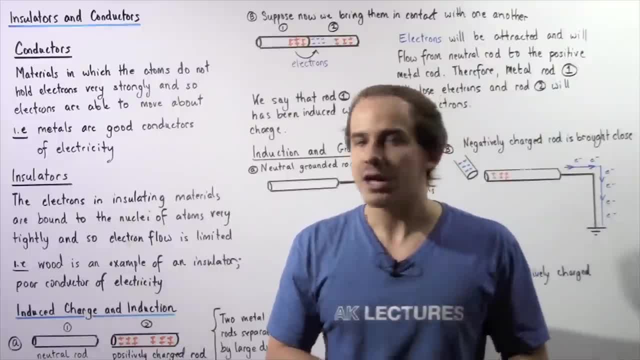 from the area where we have more, from the area where we have more electrons to the area where we have less electrons, to the area where we have less electrons, to the area where we have less electrons. and that means electrons will electrons, and that means electrons will electrons, and that means electrons will begin to flow from the neutral rod to. 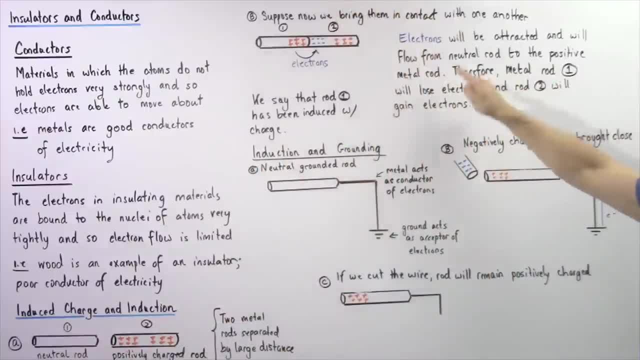 begin to flow from the neutral rod, to begin to flow from the neutral rod to this positively charged rod. so this positively charged rod, so this positively charged rod, so electrons will be attracted and will electrons will be attracted and will electrons will be attracted and will flow from the neutral rod. rod number one: 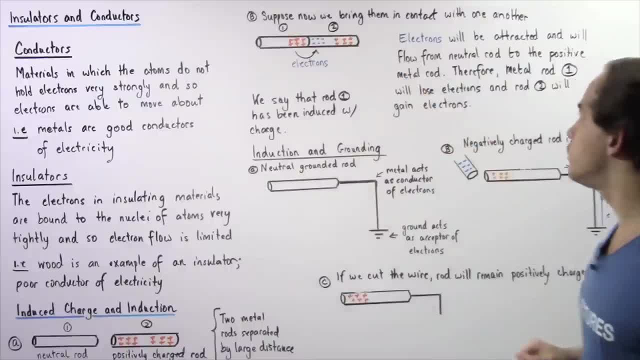 flow from the neutral rod rod number one. flow from the neutral rod rod number one to the positively charged rod rod number. to the positively charged rod rod number. to the positively charged rod rod number two. therefore, metal rod number one will. two, therefore, metal rod number one will. 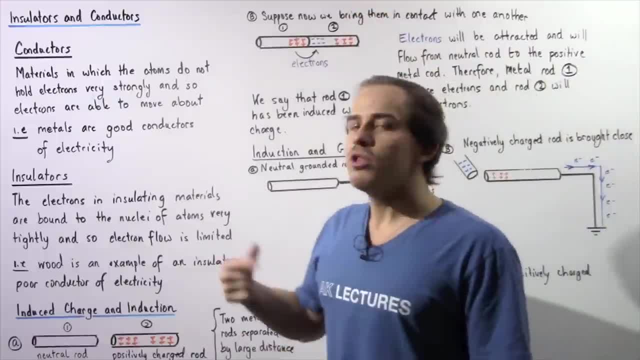 two. therefore, metal rod number one will lose electrons and rod number two will lose electrons and rod number two will lose electrons and rod number two will gain those electrons. so we say that rod gain those electrons. so we say that rod gain those electrons. so we say that rod number one has been induced with a. 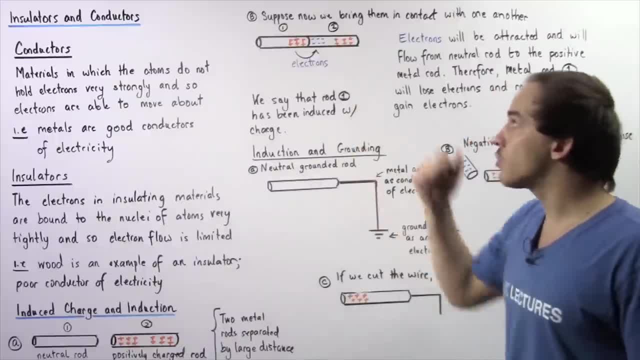 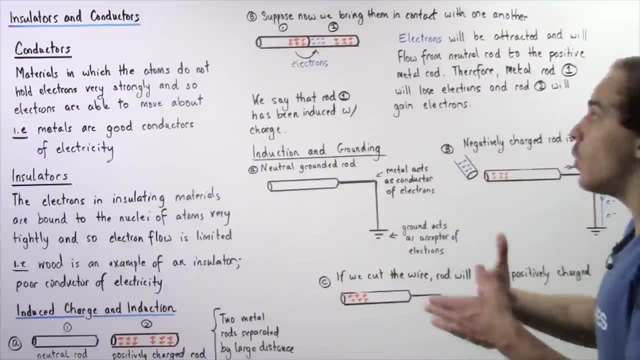 number one has been induced with a number one has been induced with a charge. and this process of charging our charge and this process of charging our charge and this process of charging our rod is known as induction. now another rod is known as induction. now another rod is known as induction. now another type of induction exists in which we 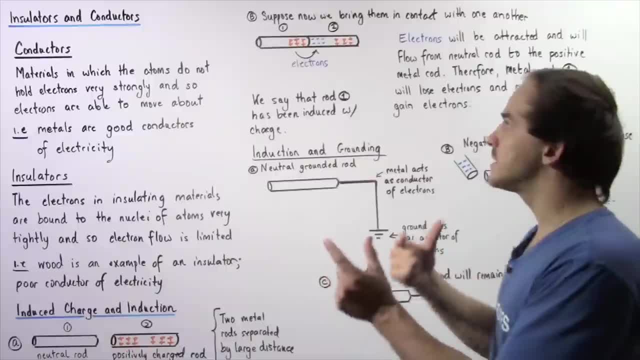 type of induction exists in which we type of induction exists, in which we don't actually have to bring these two, don't actually have to bring these two, don't actually have to bring these two objects in physical contact with one, objects in physical contact with one another. so let's examine induction and 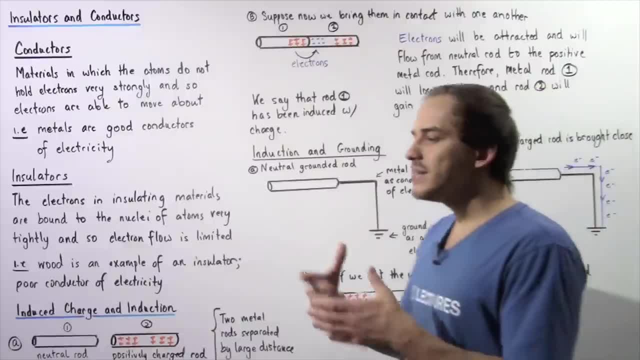 another. so let's examine induction, and another. so let's examine induction and grounding. so whenever we ground an grounding, so whenever we ground an grounding, so whenever we ground an object, we essentially connect that object, object, we essentially connect that object, object, we essentially connect that object to the ground. so we take a wire, we take 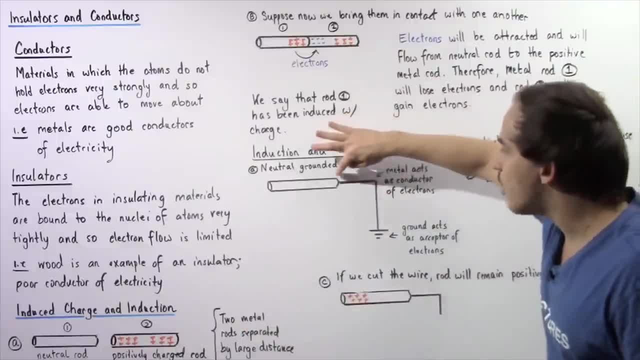 to the ground. so we take a wire, we take to the ground. so we take a wire, we take some type of conducting material and we some type of conducting material and we some type of conducting material and we connect our rod to the ground. so this is connect our rod to the ground. so this is. 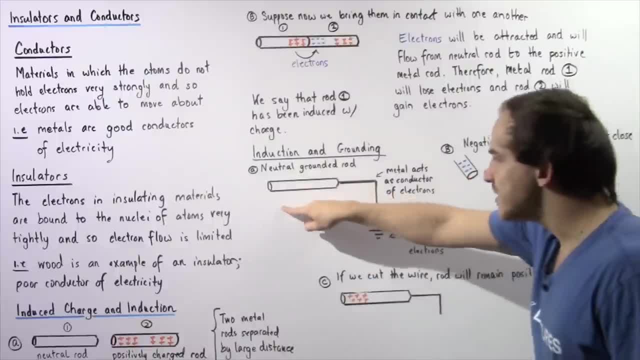 connect our rod to the ground. so this is a symbol that means grounded. so this is a symbol that means grounded. so this is a symbol that means grounded. so this is a neutral rod and we connect our rod to a, a neutral rod and we connect our rod to a. 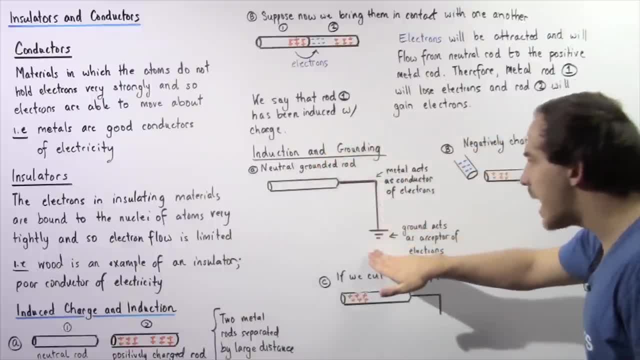 a neutral rod and we connect our rod to a metal wire and that metal wire is metal wire and that metal wire is metal wire and that metal wire is connected to the ground. so the metal acts connected to the ground, so the metal acts connected to the ground, so the metal acts as a conductor of electrons and it. 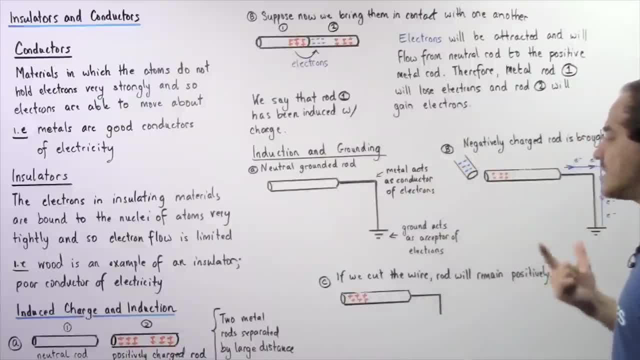 as a conductor of electrons and it as a conductor of electrons, and it allows the flow of electrons and the allows the flow of electrons and the allows the flow of electrons and the ground acts as an acceptor of those. ground acts as an acceptor of those. 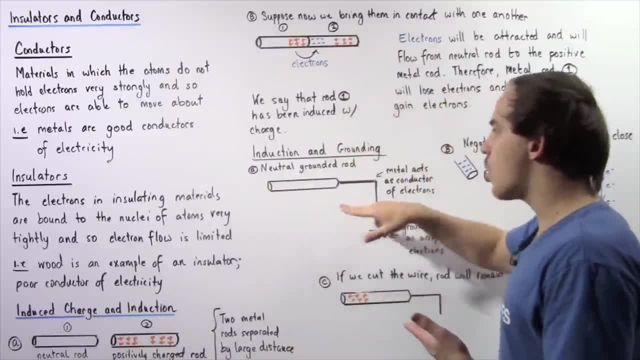 ground acts as an acceptor of those electrons. so once again we have a neutral electrons. so once again we have a neutral electrons. so once again we have a neutral charge. so let's suppose we move on charge. so let's suppose we move on charge. so let's suppose we move on to Part B. in Part B we bring a. 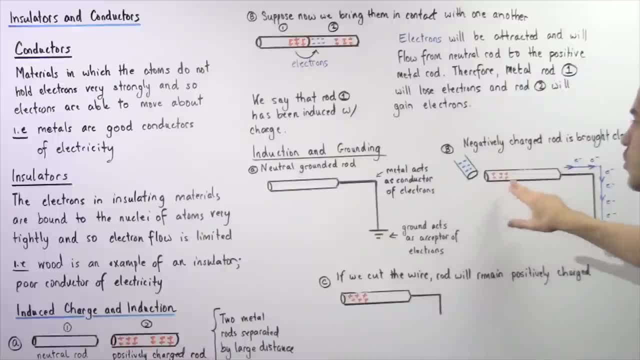 to Part B. in Part B, we bring a to Part B. in Part B, we bring a negatively charged rod very close to negatively charged rod, very close to negatively charged rod, very close to this rod. what will begin to take place? this rod. what will begin to take place?